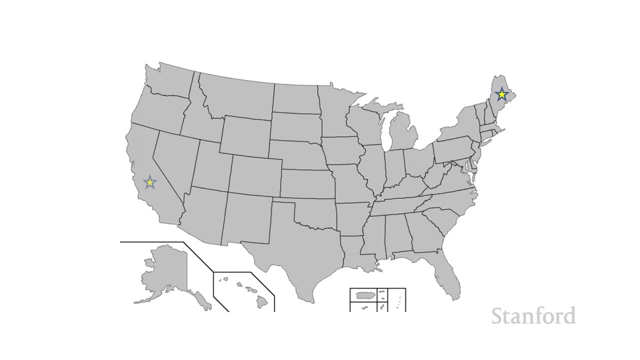 wants to buy one of my toys, And so what do I do? Well, here's a possibility: I hire a truck And my truck takes the toy out to a train station And we transfer the toy to the train station And the train goes to Chicago. 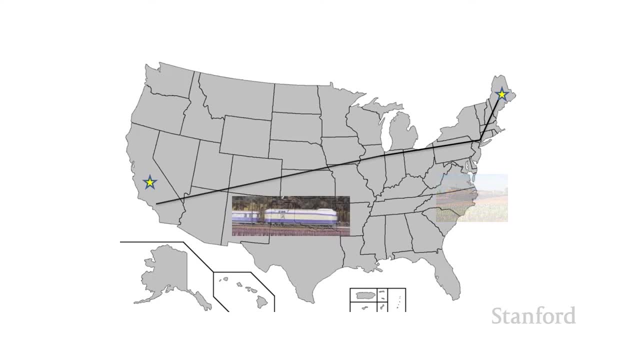 And then it transfers to another train And that ends up somewhere in Los Angeles And then I hire another truck to take the toy from Los Angeles out to wherever my former student's living. So this will get the toy to my former student, Assuming I can manage the complexities of running. 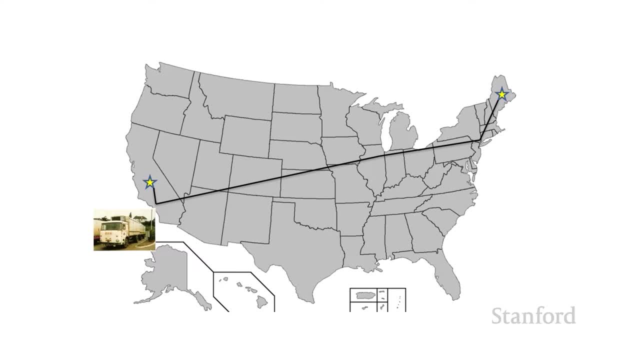 an entire transportation network, But this doesn't seem like a very good idea, does it Now? I don't want to do this. I want to concentrate on building the toys. I don't want to deal with any of the transportation stuff. 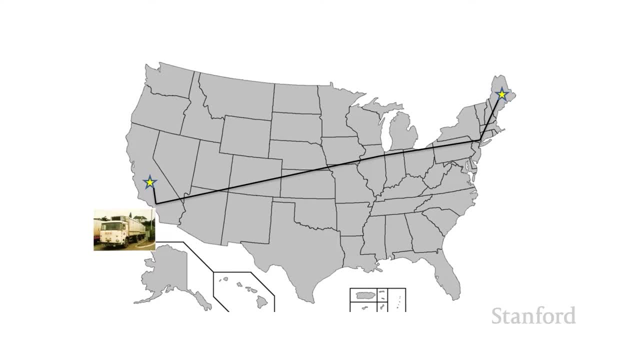 What I'd like to do is I like to take the toy and drop it off at the FedEx office and magically have it appear at my former student's house. Now, all the steps that I previously attempted to go through, like hiring trucks. 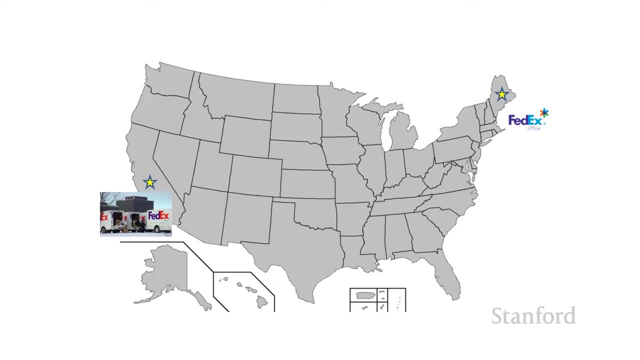 working out train schedules, filling trucks with gasoline. that all still happens, But the difference is- I'm not dealing with it, FedEx is, And so the same sort of process occurs when we're developing software for the internet. Ultimately, there are people that 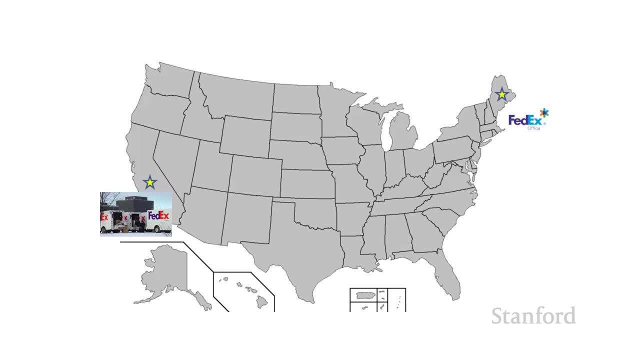 do work at that bottom layer, at the layer where somebody's trying to figure out how to fill up the trucks or working out the train schedules. But most programmers don't. They don't know how to do it. They don't know how to do it. 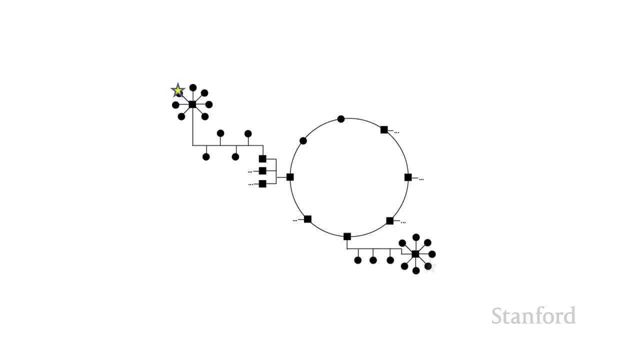 They don't know how to do it. Most programmers programming applications on the internet don't deal with that level of complexity. Instead, they do the equivalent of dropping off some information at the FedEx office and having it magically appear on the other end. 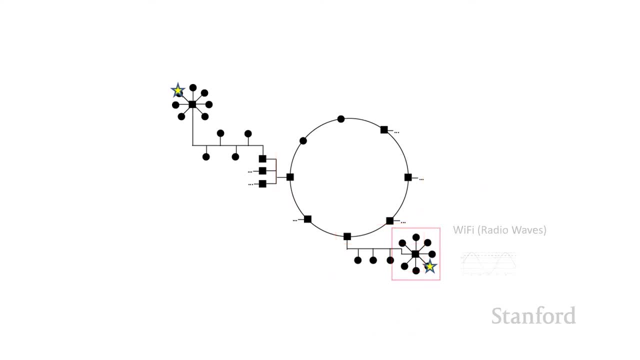 So what we're going to do is we're going to take a look at what's sometimes referred to as the internet protocol stack And we're going to take it from the bottom layer, that filling the truck up with gas layer, where the rubber really 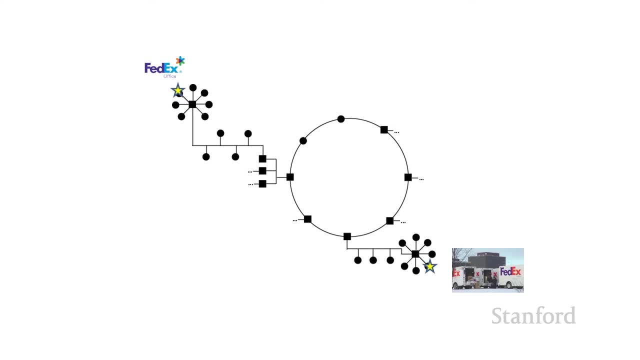 hits the road and we're going to see the different layers That are built on top until we get up to the top layer, which is where the applications happen, where they do the equivalent of dropping information off of FedEx and it magically appears on the other end. 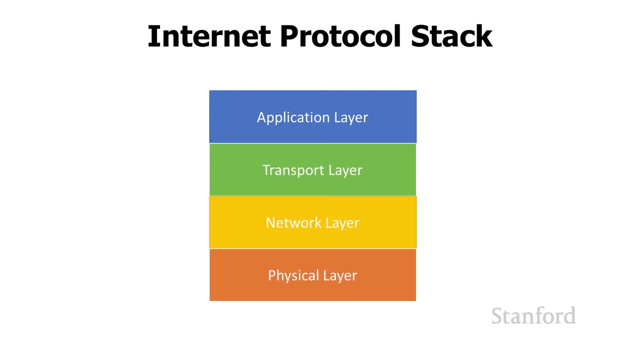 All right, so this is the internet protocol stack. Then, at the bottom layer, we have the physical layer, And that's the layer, basically the level where we're filling the truck with gasoline, And then we have a number of layers on top of that. 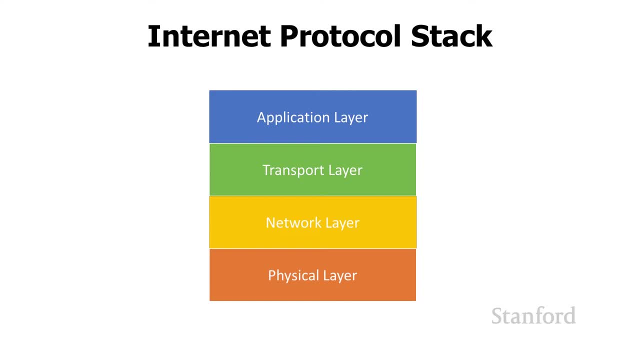 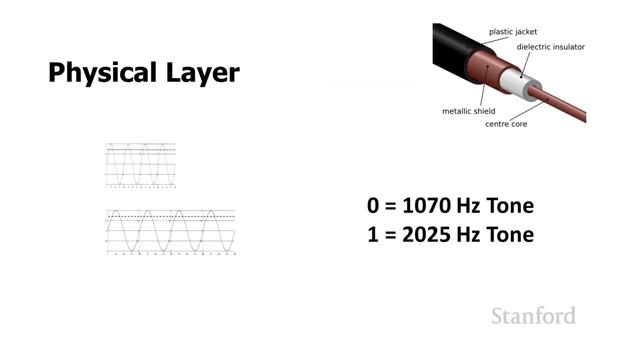 And then, at the top layer, we have the application layer, And that's the layer where people are just dropping packages off of FedEx. So let's take a look at each of these layers and see how they work. The first layer, the bottom layer, is the physical layer. 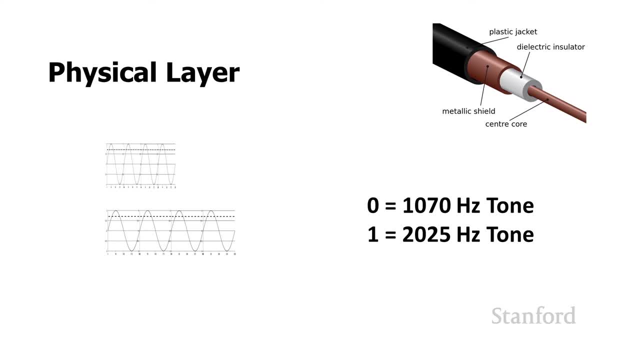 When we're working at the physical layer, we need to decide exactly how we're transmitting information to using 0s and 1s. So, for example, when we're transferring information over the telephone, are we going to have a 1070 hertz tone. 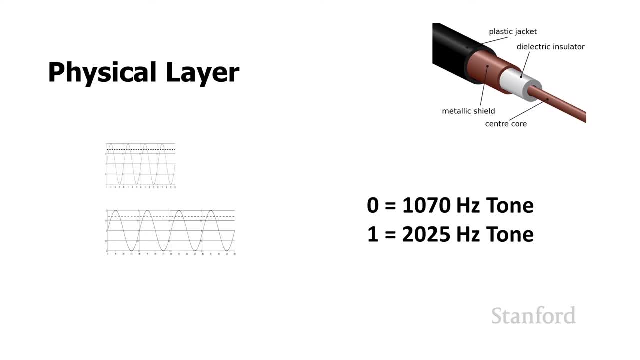 or are we going to have a 2025 hertz tone, and which one of those is going to represent 0, and which one of those is going to represent 1?? We need to figure out what the physical connections look like. We need to figure out how everything's. 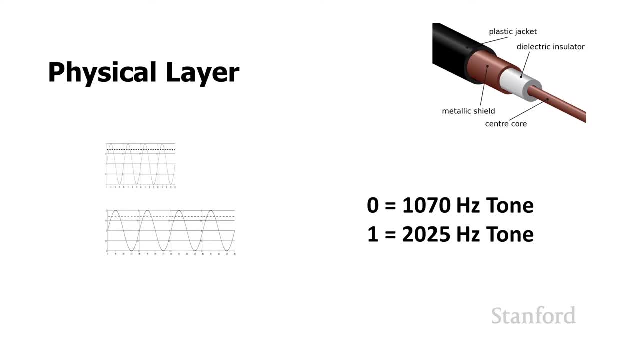 going to fit together. Now, the thing about the physical layer is: anytime you come up with a new network, you are going to have to define a new physical layer, And we're going to find that this is not the case with all the layers. 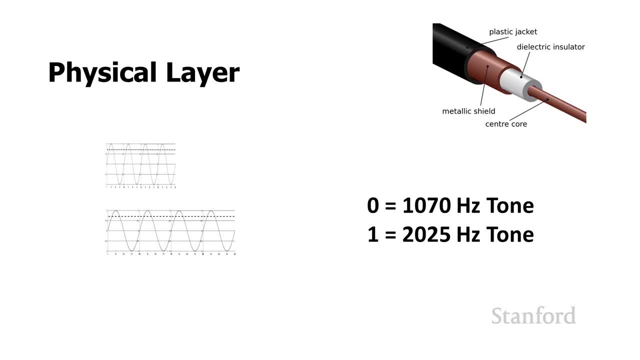 But the lower layers we need to define a new copy of every time we have a new type of network. So if I decide that the best way to get information across the Pacific is to have a bunch of sharks with frickin' laser beams on their head, that 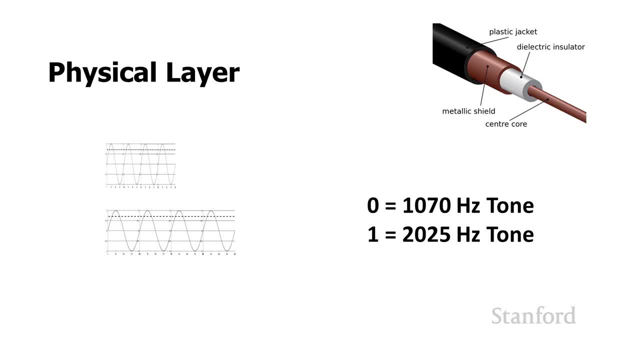 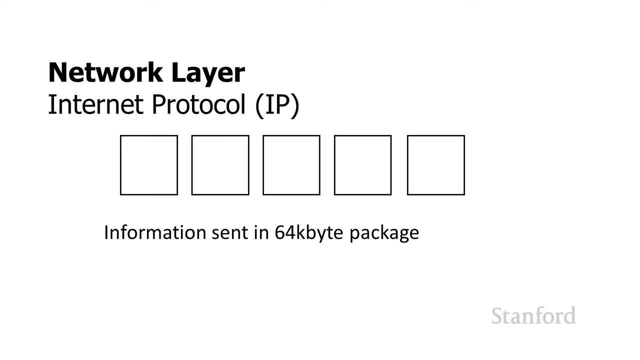 I need to figure out how those sharks are going to transmit 0s and 1s across the Pacific. On top of the physical layer is a network layer. The protocol at the network layer is the internet protocol. This is the same internet protocol. 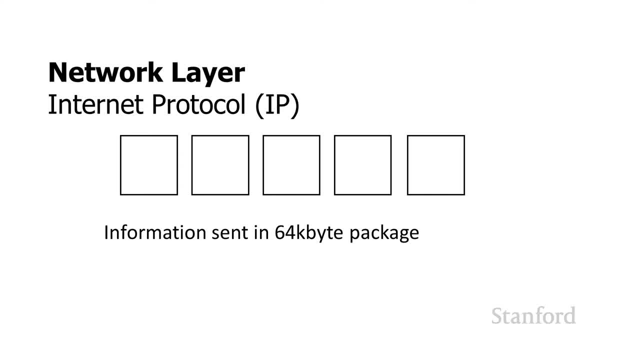 that we saw when we were seeing IP addresses. While this layer is built on top of the physical layer, it's still quite primitive. All information sent with the internet protocol is going to be limited to 64 kilobyte packets, And these packets will include the IP address of the sender. 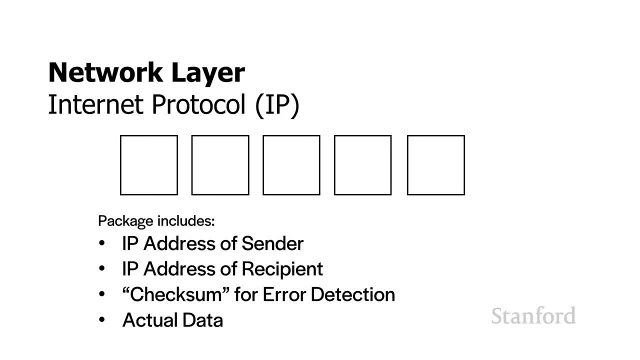 the IP address of the recipient, a checksum, which is a means of trying to determine if something accidentally messed with some of the bits in the packet, and then the actual data, One of the things that particularly makes this network layer a bit annoying to work with. 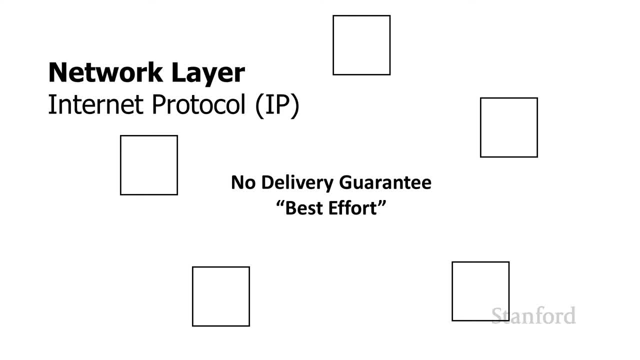 is there's no delivery guarantee. The internet protocol layer says it will make the quote best effort, end quote to get the package to the destination, And so one of the questions is: why do we have this really primitive layer? And the answer is because, again, 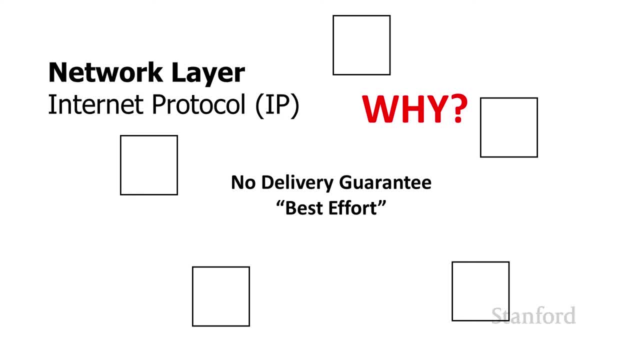 any time we have a new type of network we want to define. we need to define the physical layer and we need to define the network layer. So, going back to my sharks with frickin laser beams, example, I need to get those sharks to somehow line up. 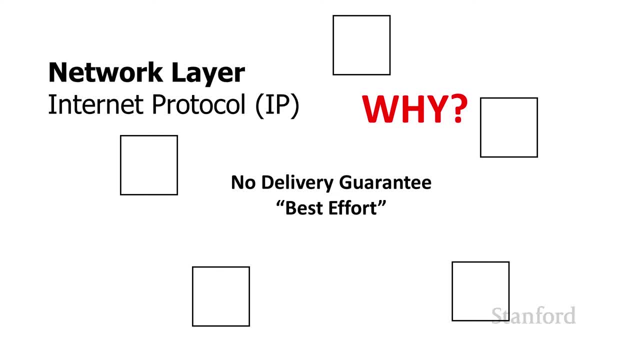 to get packets from one side of the Pacific to the other side. I don't want to deal with a more complex protocol. I want the simplest protocol possible because I'm having enough trouble just trying to get these sharks aligned. So because the network layer is relatively simple. 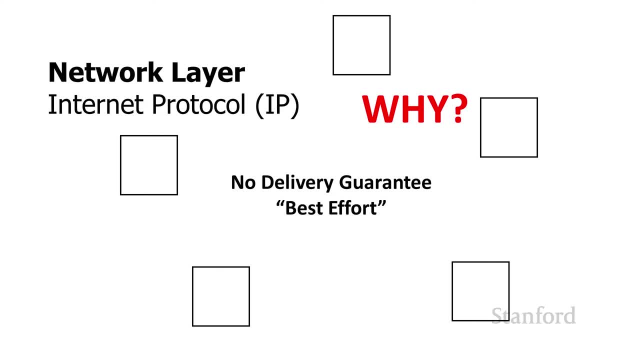 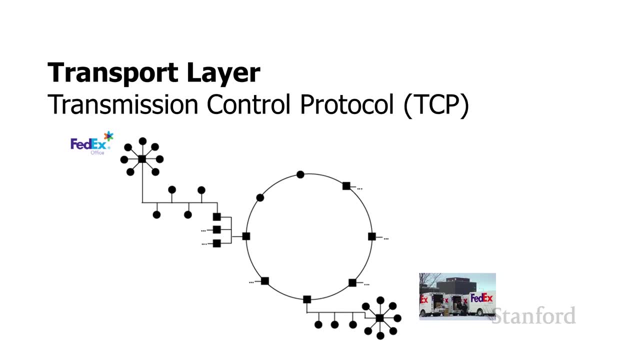 it's going to be relatively easy for somebody to come up with a new network type and implement the network layer on that new network type. Going up a layer, we have the transporter layer. There's actually several protocols that work at this layer, but by far the most famous. 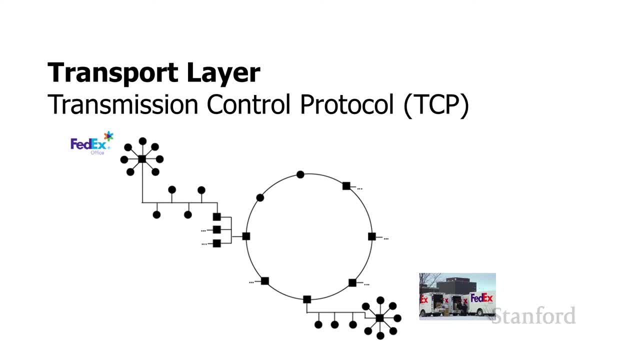 is the transmission control protocol, or TCP. The TCP protocol basically acts as our FedEx does. What we're going to be able to do with the transmission control protocol is it's going to build on top of the network layer and, ultimately, on top of the physical layer. 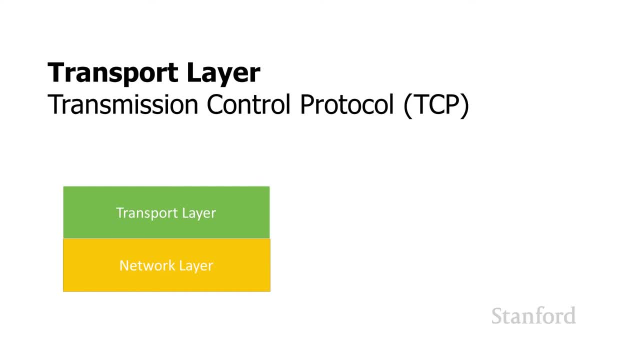 And we're going to be able to just drop off packages at the transmission layer and they will magically appear at the other side. TCP and IP are often considered the key internet protocols, the most important protocols of the internet. Let's take a look at how these two work together. 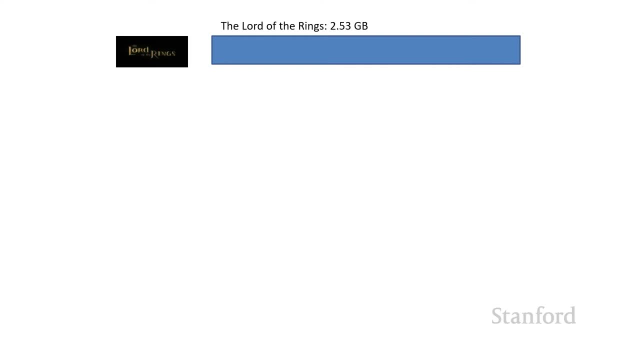 to get their job done. So what we have here is a video of the Lord of the Rings, the Fellowship of the Ring. It's 2.53 gigabytes and that actually means I made this little interactive video back before we had high definition televisions in widespread use. 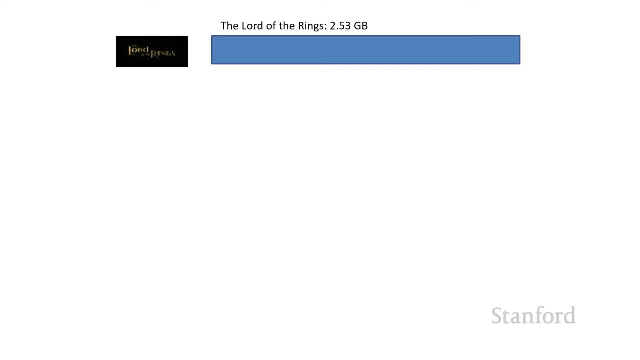 So at 2.53 gigabytes, this movie is too large to fit into our individual 64 kilobyte packet. So if we want to send this movie, what needs to happen is it needs to be divided up into all these little packets. 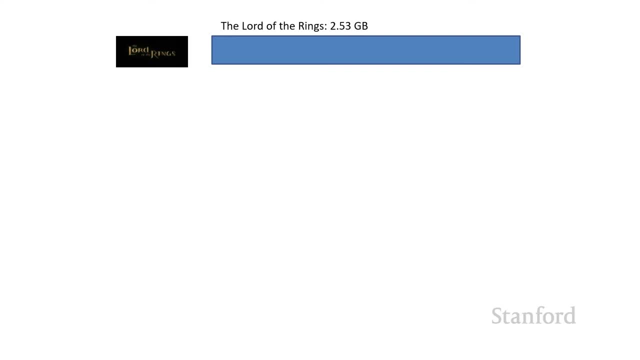 And this is something That TCP is going to do for us. So, as somebody who's building on top of TCP, I hand the movie to TCP. TCP breaks the movie down into all these little individual packets And, if you work it out, there are over 663,000 packets. 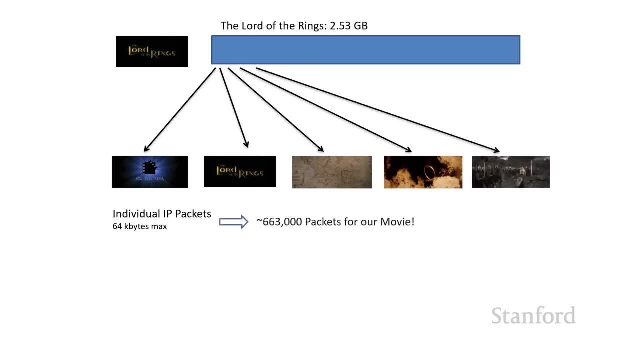 for the entire movie. What TCP is going to do is it's going to number each of the individual packets And it's going to mark the packets with the IP number of the source computer and the IP number of the destination computer. OK, All right. 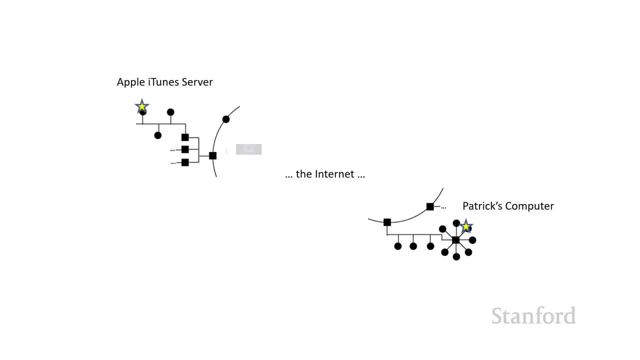 It is then going to start sending the packets through the internet using the internet protocol. As we previously discussed, the internet protocol does not guarantee transfer. It just makes the best effort. Among other things, this means some packets will get lost and some packets will arrive in the wrong order. 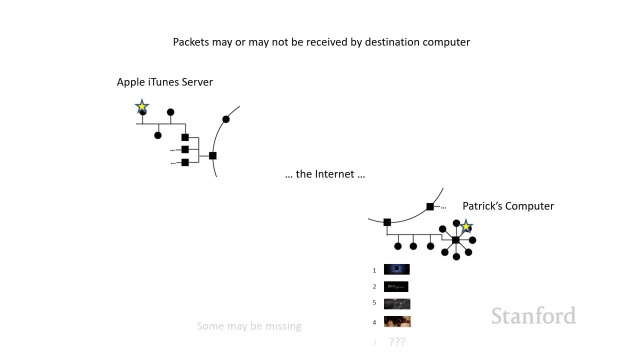 Now, what TCP is going to do is it is going to keep track of the different packets. If the packets arrive in the wrong order, it's going to reorder them to the correct order And, even nicer, it's going to keep track of the total number of packets. 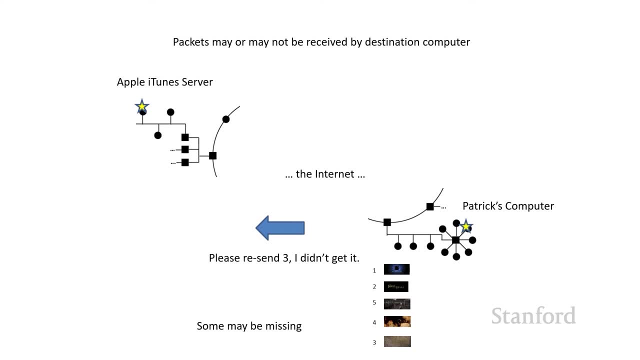 And if some of the packets are missing, it will send a request using IP back to the original computer saying: hey, that packet didn't show up, Can you send me another copy? And then that copy will get sent over From the point of view of somebody who is using TCP. 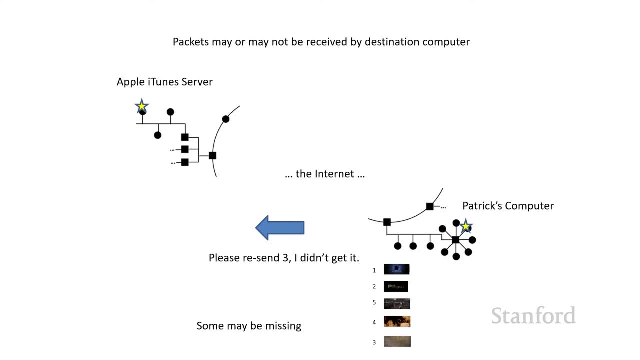 this is all completely hidden. As far as the user of TCP is concerned, we just have a direct connection from one computer to the other computer. We can shovel whatever information we want into this connection and it will magically appear on the other side. 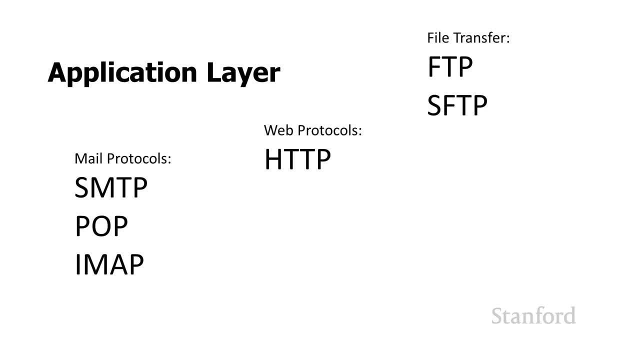 Finally, that brings us to our last layer, the application layer. This is the layer where all the stuff you guys care about happens. So we have a whole bunch of mail protocols: SMTP, POP, IMAP. The protocol for the web HTTP is here. 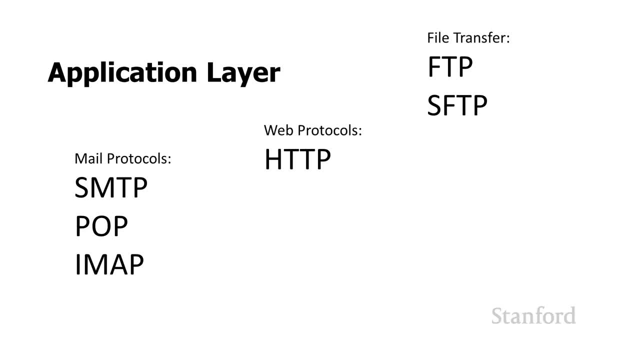 There's file transfer protocols like FTP and secure FTP, And basically every program That is on the network that does anything needs to have some sort of a protocol. They may be well-specified protocols that are publicly available and that different programs can interoperate with, or they may be completely proprietary. 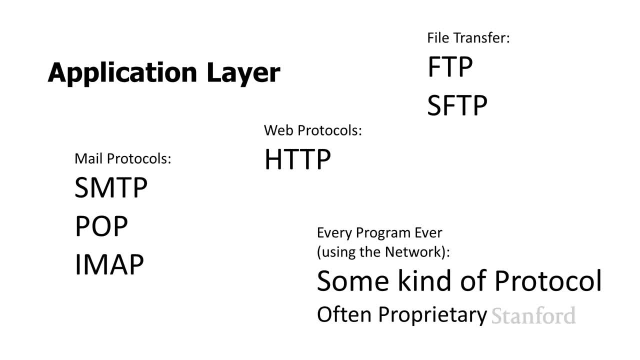 But ultimately, as we've seen previously, if two computers are on the network and are operating together, there needs to be some sort of formal agreement between those two computers, And that formal agreement is a protocol, But, as we've seen, the application layer. 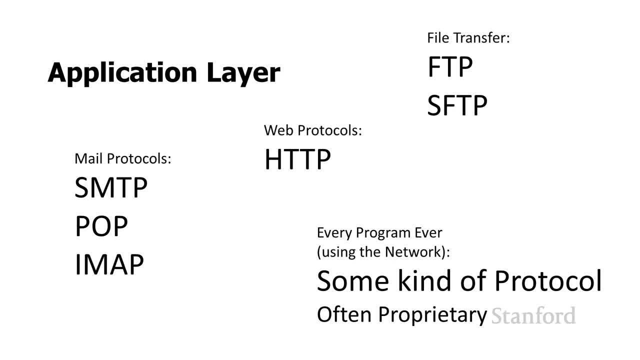 is built on top of the other layers. So if you come up with some great cool new idea for a brand new type of application on the internet, you do not have to go back and say, hey, I need to figure out how to move those packets around. 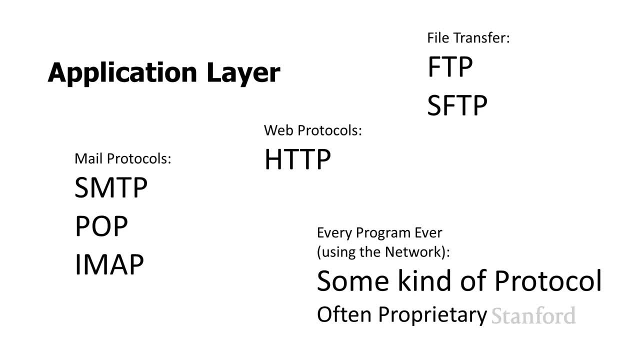 I need to know how to reorder those packets. That is completely handled for you by TCP. You're just going to hand things to TCP and TCP will take care of that. You do not have to worry about. hey, am I running this? 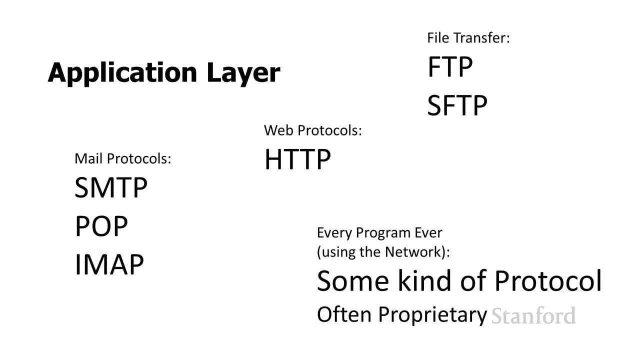 over a Wi-Fi network? Am I running this over fiber optic cable? Am I running this over? Or Patrick's sharks with frickin' laser beams network? That is all completely hidden by the lower layers, So you can see that this layer protocol really. 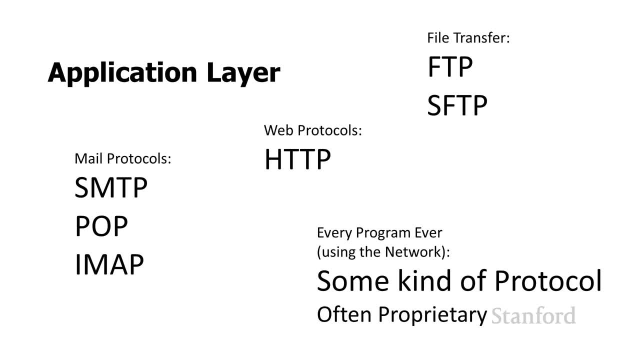 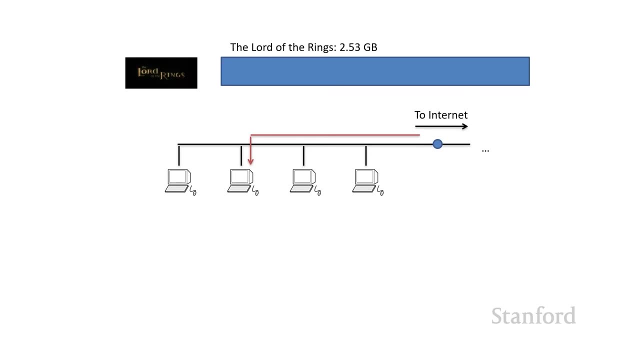 provides some great advantages to the people on the top layers. There are some other handy implications of the fact that everything down below is handled by packets. Consider, for example: I'm sitting in my dorm room and I'm trying to download the Lord of the Rings. 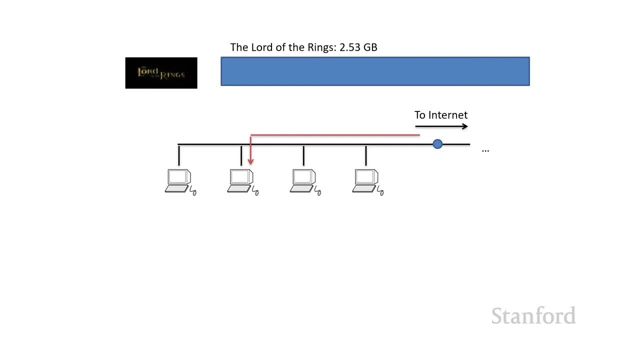 Now it turns out that all Internet traffic from our particular floor travels through the same cables to the wider internet for the university, And so without packets. while I'm downloading the Lord of the Rings, nobody else can do anything, But because the traffic is broken down into packets. 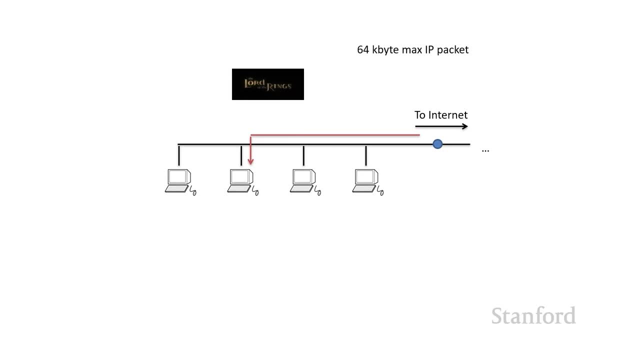 what's going to happen is: I will get my little 64 kilobyte packet from the Lord of the Rings. Maybe my friend next door is watching the movie Up. She'll get her 64 kilobyte packet from Up. I'll get a packet from the Lord of the Rings. 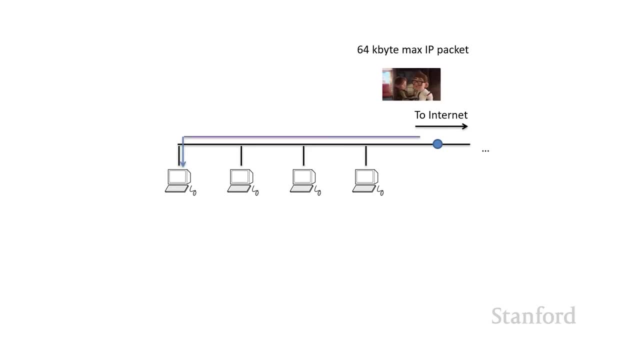 Maybe somebody is actually trying to get some work done. They'll get some email in And basically the packets will all be sharing the same cable And some packets will come in for me, Some packets will come in for somebody else. People will be able to get work in between our packets. 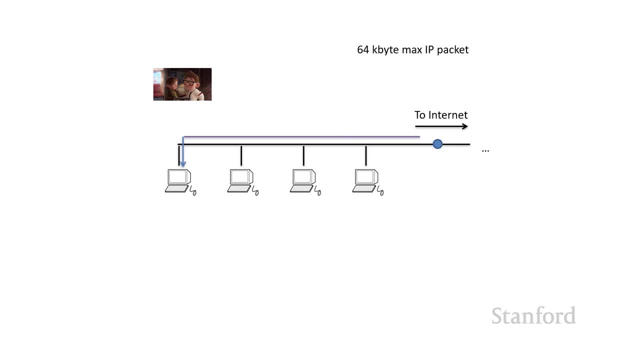 And again, if we were to send everything in just one large chunk, maybe you'd get the same amount of traffic through, But everybody would have to sit around and wait for that big chunk to come through. So the fact that things are broken down into packets- 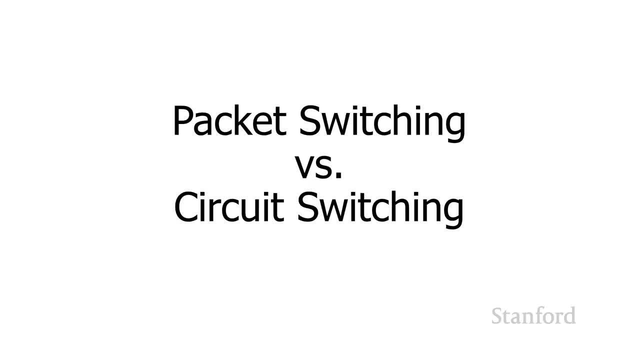 is actually pretty great. Another situation which packets work really well is when they're being used for communication purposes. So if you look into telecommunications, you'll discover that there's two different ways that telecommunications can happen. You can either have what's called circuit switching, which 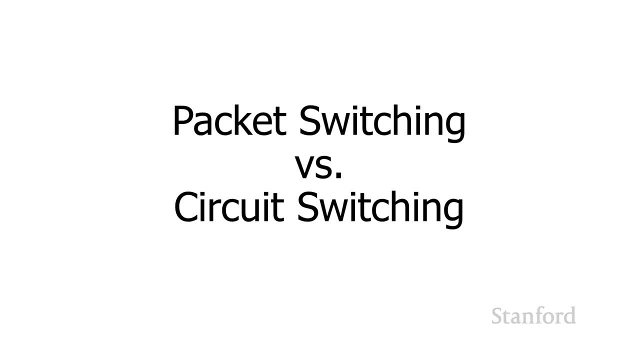 is traditionally how telecommunications has happened. or you can have packet switching And actually everything's been moving to packet switching. You may have noticed that the telephones at Stanford or often Cisco phones. you may think I thought Cisco was a networking company. 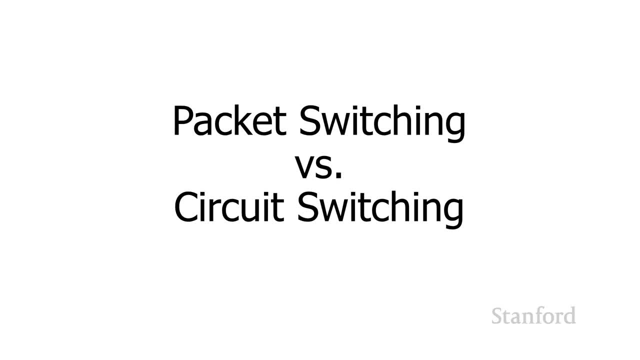 I didn't think they were a telephone company. Well, we're using Cisco phones because the Cisco phones use internet packet technology, And it turns out internet packet technology is just much more efficient than traditional telephones. So let's take a look at how this actually works. 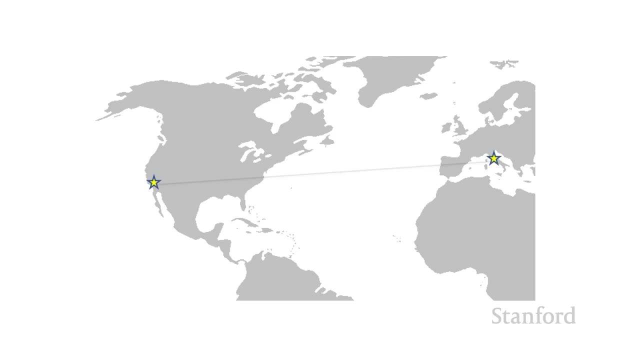 So I've mentioned my friend Tammy several times, And she moved to Italy a long while back And And so we would talk on the phone And using traditional circuit switching technology, what happens is, when I'm on the phone talking to Tammy, 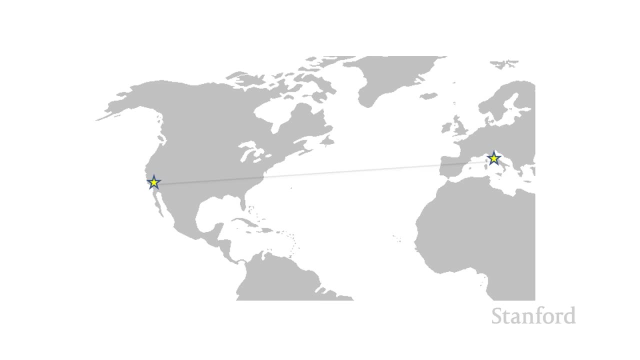 there is a dedicated line between Stanford and Italy, And so it may not be a single line. It actually is a series of lines going through different switching stations, But ultimately, all along the way, there is a specific wire. while I'm on the phone with her, 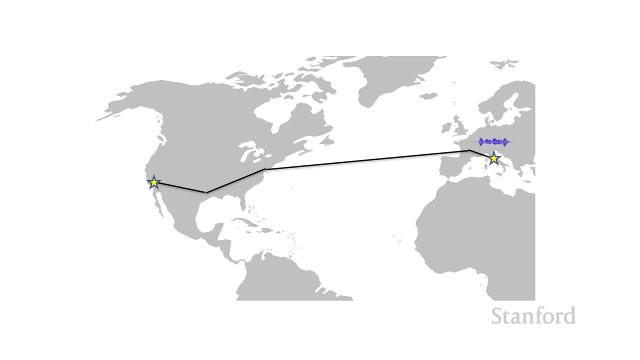 completely dedicated to the two of us. OK, And if we're talking, it's going great, We're using our wire. And if we're mad at each other and not saying a whole lot, well, those lines are still completely dedicated to us. 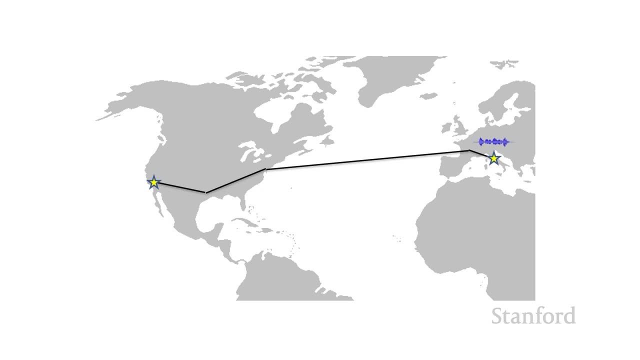 even though we're not saying anything. So this is not necessarily the most efficient use of these wires or these cables that are connecting Stanford to Italy. Now you may have noticed that most of the calls that some of you have been making to friends overseas- 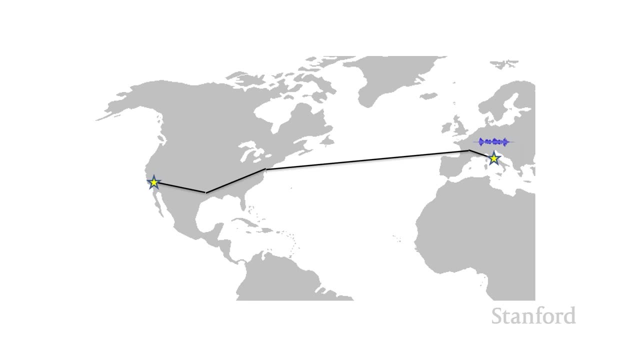 is actually completely free. Maybe you're using something like FaceTime or Google Hangouts or something like that. Those technologies use internet packets, And so what's happening in those situations is, instead of you having a completely dedicated circuit between you and say: your friend in the Bing Overseas. 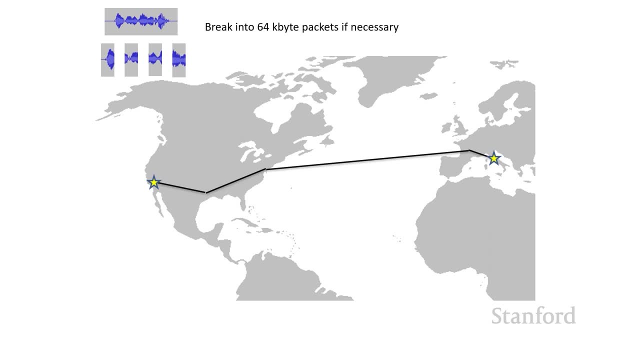 program in South Africa. what's happening is your voice is being chopped up into these little 64 kilobyte packets. Those packets are being shoved into the network along with everybody else's packets And your packets are going to arrive out on the other end. 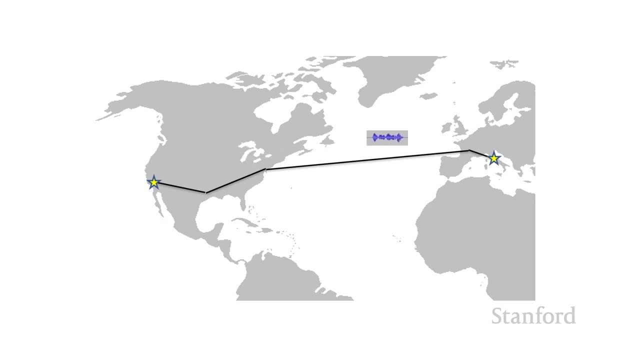 And because the lines are now shared, it's not as expensive as when the lines were dedicated. And to be perfectly honest, the telephone system between here and Italy was not so great that having a dedicated line necessarily led to great results anyway. So maybe FaceTime is for the best. 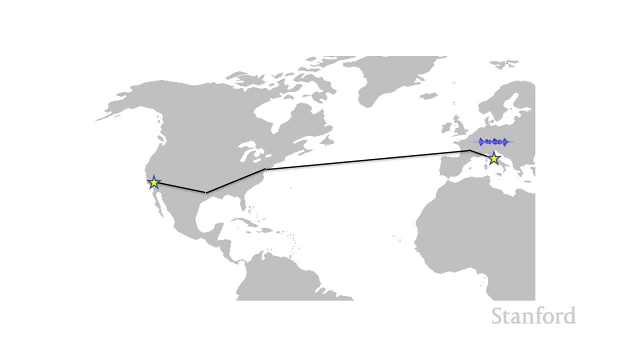 Yeah, Yeah, Although I have had not so great experiences using Skype to people out in South Africa, So a lot of it depends on how the internet connection is going. And that actually brings up another interesting point about how the whole packet situation works. 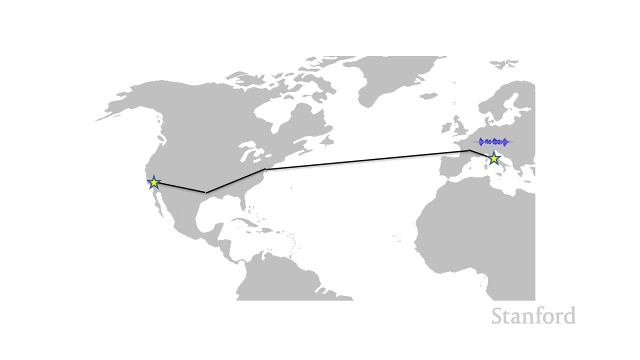 Because the packets are being shared on the line with everything else. sometimes the packets get bottled up along with the rest of the internet traffic, And so what's happening is, on the other end, you're receiving a bunch of packets and you have to decide: gee, I'm missing this packet. 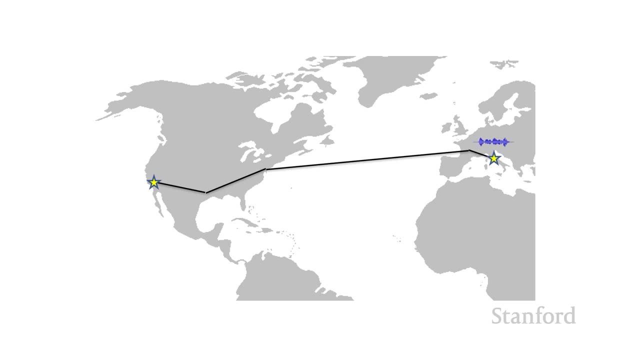 But if I wait too much longer before playing the video, my user is going to think this is getting a little bit weird, So maybe I should go ahead and play the video before that packet arrives, and we're just going to have a glitch. 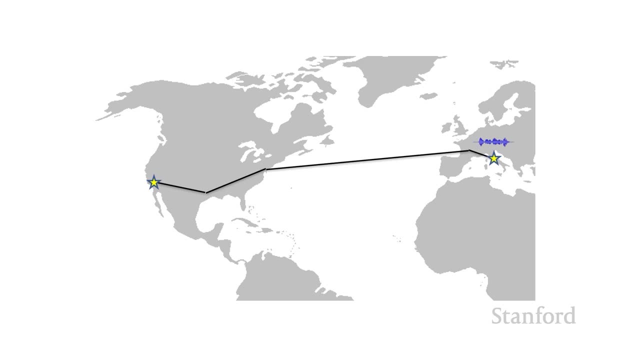 So there's all sorts of interesting situations that can occur because this information is being sent in packets. All right, That's it for our study of the internet and the internet protocol. Where we're going to move to next week is we're going to start looking at the World Wide Web. 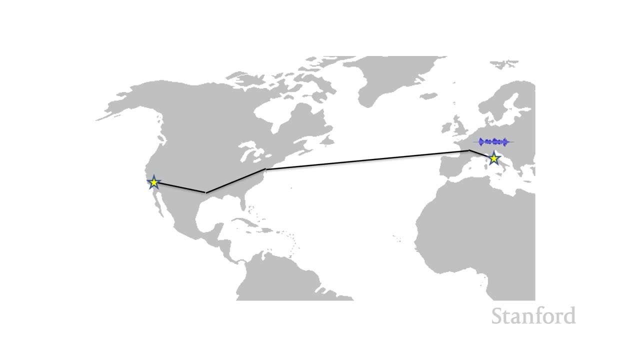 and we're going to start learning how to make web pages. I'll talk to you soon. Have a great weekend.